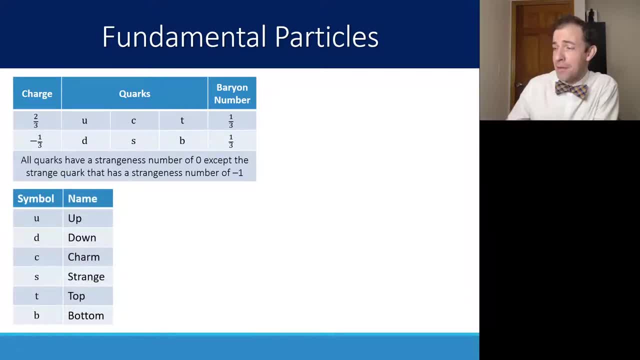 down- charm, strange, top and bottom, represented by the symbol shown here. The table that's given to you in the IB physics data booklet is shown up here. You'll notice that up- charm and top quarks all have a charge of two thirds and down- strange and bottom quarks all of a charge of negative. 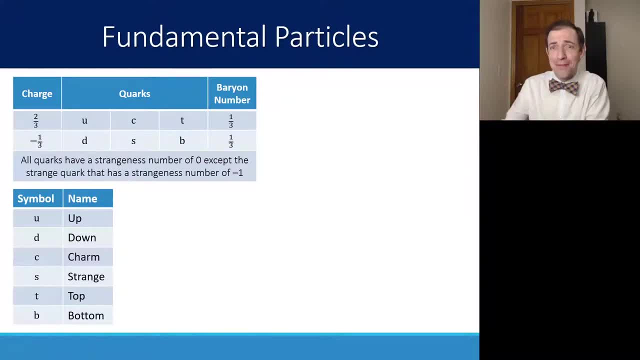 one third. Now that's going to seem kind of random, but it's not. So we're going to look at: how could you possibly have an almost full charge, And how can you have a charge that's a negative one third? Well, these quarks will always combine in either twos or threes, And when they 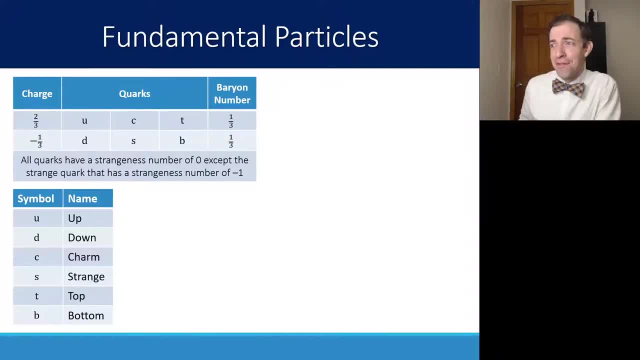 combine, you'll always get an integer number of charge, either a plus one zero or minus one charge. Now these quarks have a strangeness number to them as well, And that strangeness number is zero. So you have a strange quark that has a strangeness number of negative one. You'll also notice that 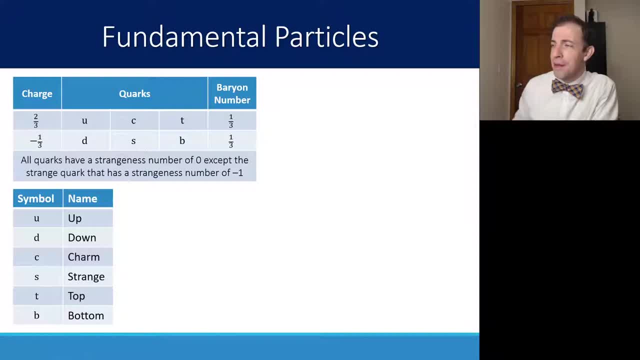 these have something called a baryon number. We'll talk about baryons in a little bit- And that baryon number for all these quarks is one third. Now there are six quarks that are shown here, but there's actually 12 quarks, because all of these quarks have an anti-quark. These 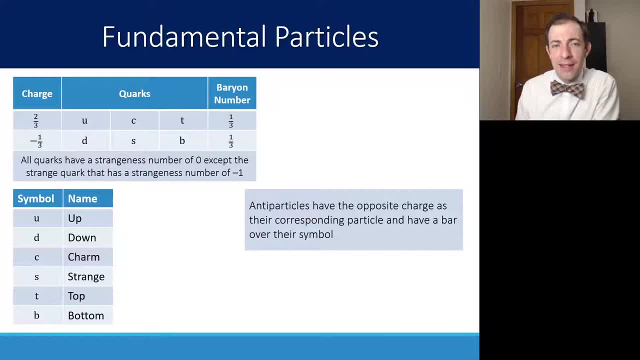 anti-particles have an opposite charge and they're corresponding as their corresponding particle and they have a bar over the symbol. So, for example, you can have a strange quark which is a negative one third, or an anti-strange quark which is just an S with a. 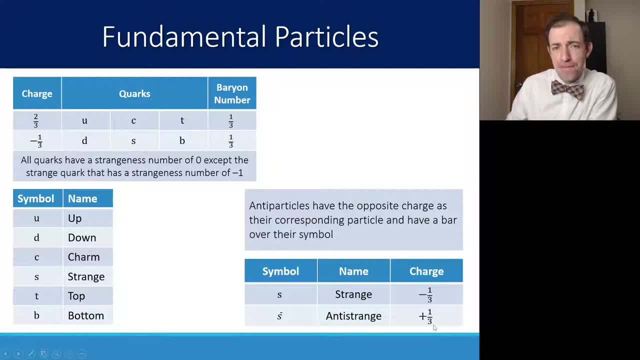 bar on the top, which is a plus one third. So you have an anti-up, anti-charm, anti-top, anti-bottom, anti-strange and anti-down. Now you also have in our list of fundamental particles the leptons. These leptons are things like the electron or the anti-electron. 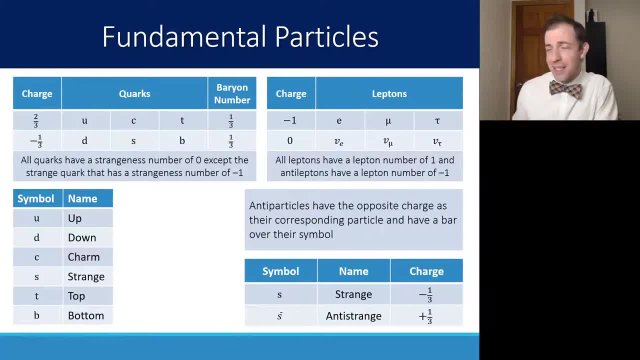 which you call the positron. Now there are other leptons as well. So in the family of electron we have the electron, the muon and the tau. These all have a charge of minus one. So you're familiar with an electron having a charge of. 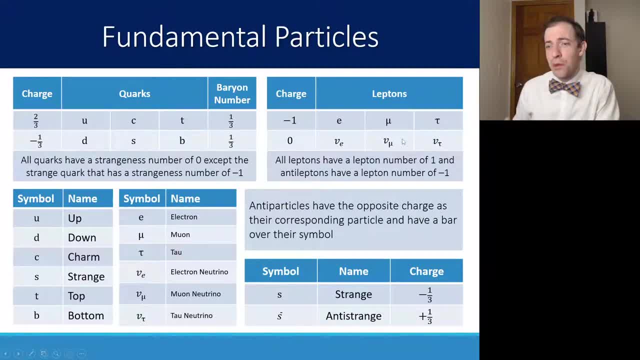 minus one. You can also have an anti- all of these which would have a charge of plus one. That'd be the anti-electron. We also call this the positron, the anti-muon and the anti-tau. 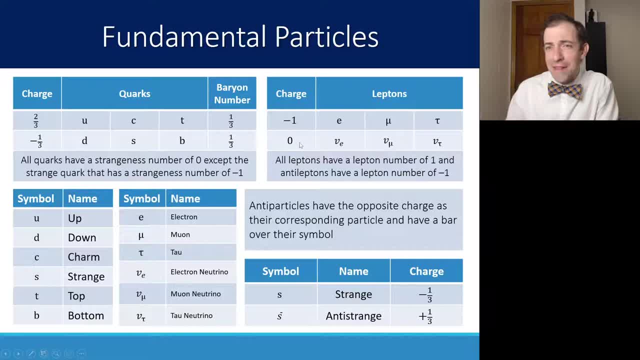 Those would all have a positive one charge. We also have these charges, These neutral particles that are leptons, called neutrinos. These are the electron neutrino, muon neutrino and tau neutrino. You'll see that subscript represented each of those different. 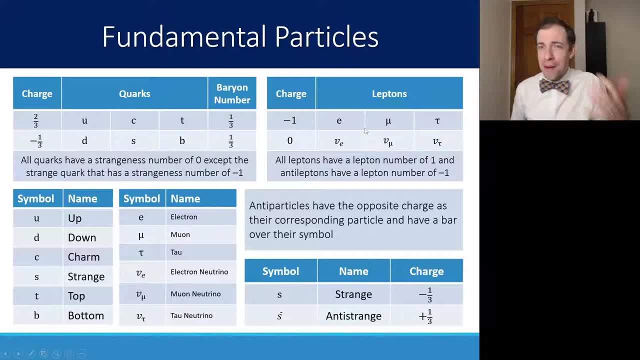 types. You can have anti-neutrinos as well. You may remember an anti-neutrino showing up in beta negative decay. All of these leptons also have a number associated with them, called a lepton number. The lepton number is one, unless it's an anti-lepton. 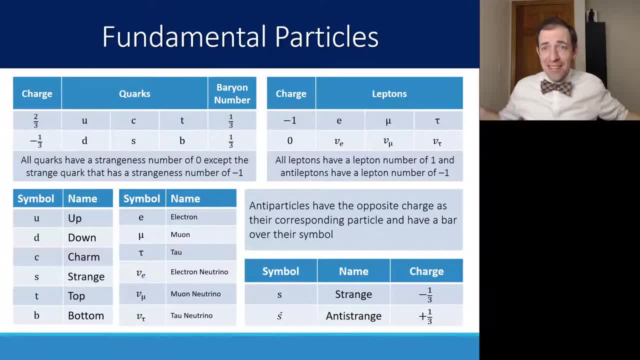 then it's an anti-lepton. If it's an anti-lepton, then it's an anti-lepton. If it's an anti-lepton, then it's a negative one. Now, that feels like a lot of different things and a lot of different things to keep track of. We will revisit this later on talking. 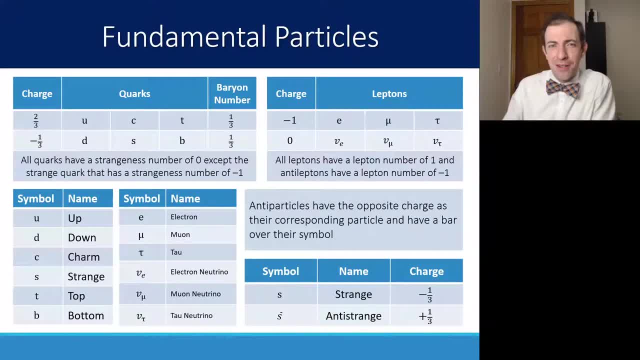 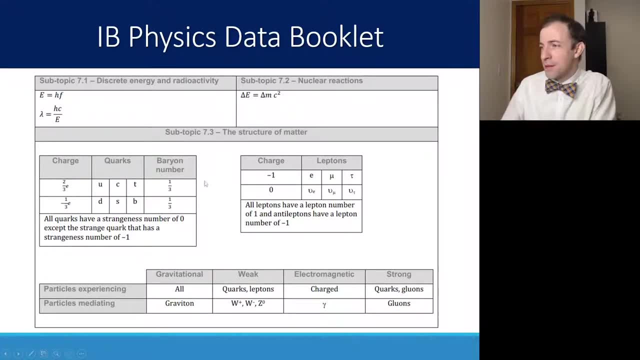 about all these different nuances and these numbers that are associated with these particles. So I want to show you what it looks like in the data booklet. It's these exact tables. They just don't look as pretty as they did in the last slide. They show up here in subtopic 7.3.. 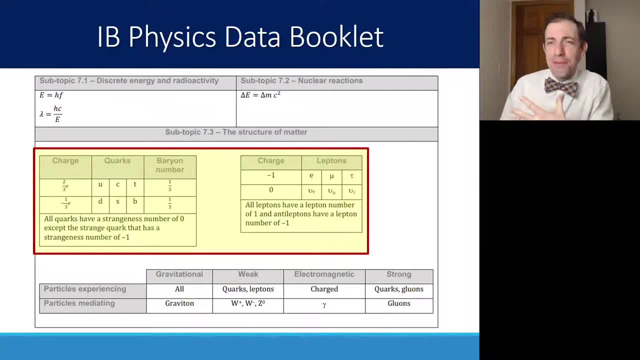 One thing that I do want to point out, something that has always bugged me in the data booklet: the charge on these down strange and bottom quarks. it has a negative in there. It's negative one-third electrons is the charge, But the negative, the way the font works out, it looks like it kind. 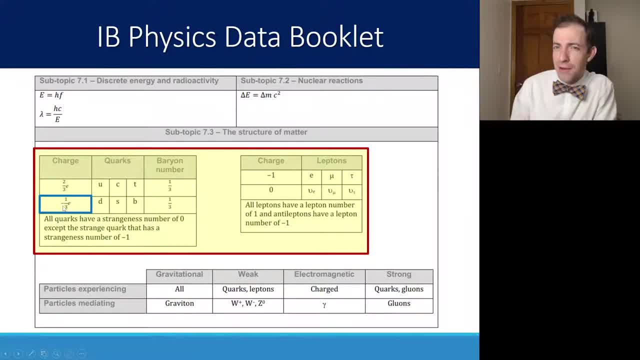 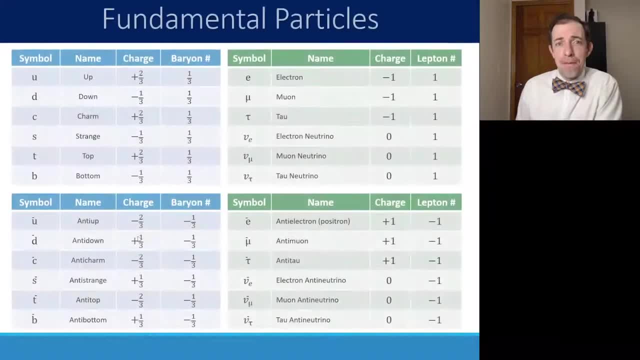 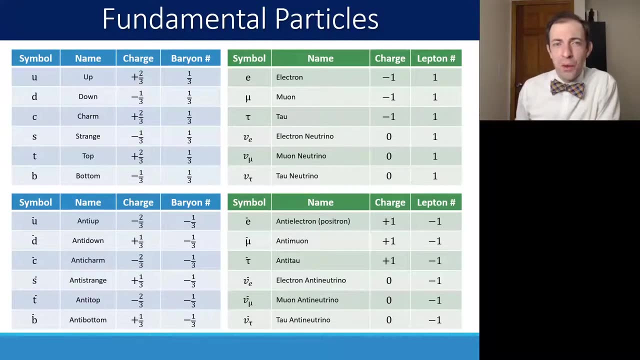 of goes in there, So it's easy to miss the negative if you're not looking for it. So just remember that it's a plus two-thirds and a minus one-third for those quarks. All right, If you really wanted to go at it, you can list from these things in the table every single one of the 24. 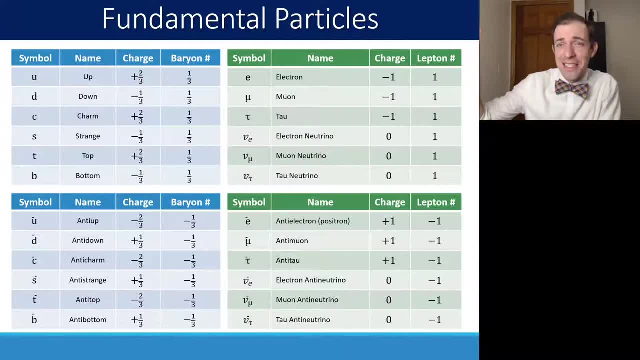 particles that we have listed with the six quarks and six leptons, as well as their anti-quark and anti-lepton pairs, And you'll see all of that kind of showing up in here with their charge and baryon number associated. All right, So that leads us to classifying particles On one side. 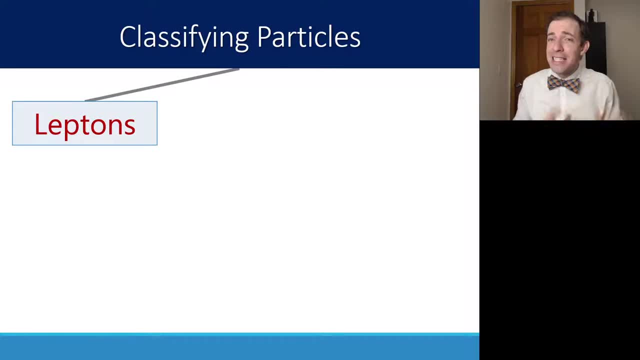 of our fundamental particles, we have these leptons. These leptons are what we just organized in that table. The common leptons that we will see is the electrons, the muons, tau, and then of course, all the neutrinos associated with those. Of course, anti-leptons are also leptons that. 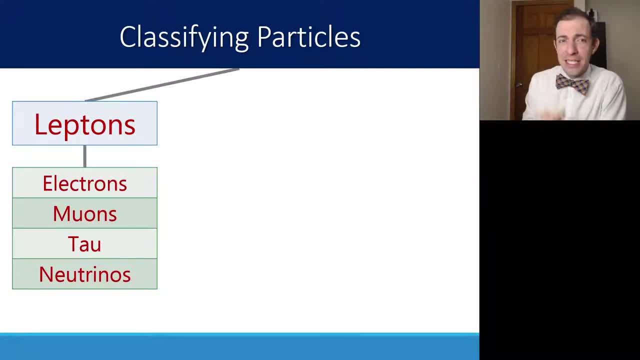 categorize in that category. there, That means that there is nothing smaller than an electron. The electrons aren't made up of any other parts to them On the other side of this tree of fundamental particles or different particles that we have in nature. 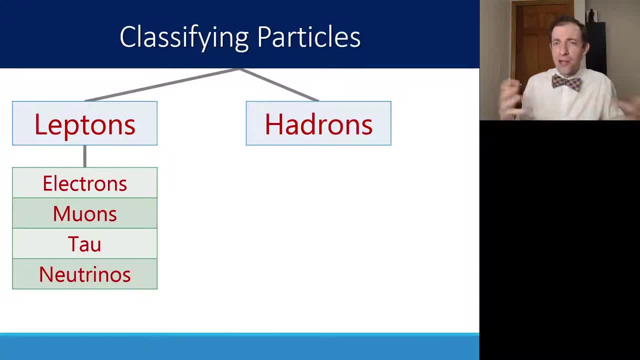 we have the hadrons. Hadrons, just like the Large Hadron Collider which you may know of, are anything that is made up of quarks. These quark-based particles can be categorized into two different sets. We have the mesons. These are things that are made out of two quarks. 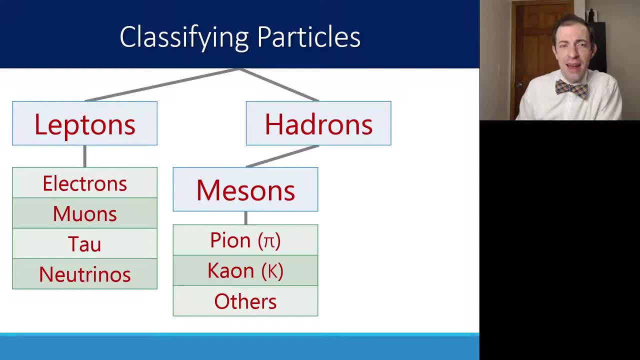 Mesons. some examples of them are the pion, the kaon and some others. There are hundreds of them, So you won't have to memorize these. You'll just be given this is a meson, Or you'll notice. 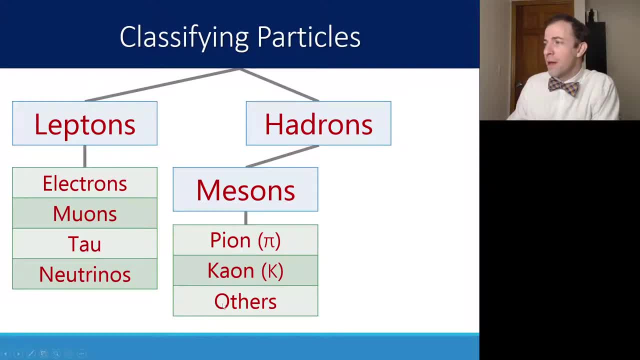 that it's made out of two quarks. That means that it's a meson as well. The other side of the hadrons, kind of under this umbrella, is the baryons. Baryons are something that you are familiar with, whether or not you realize it, because baryons include the protons and the 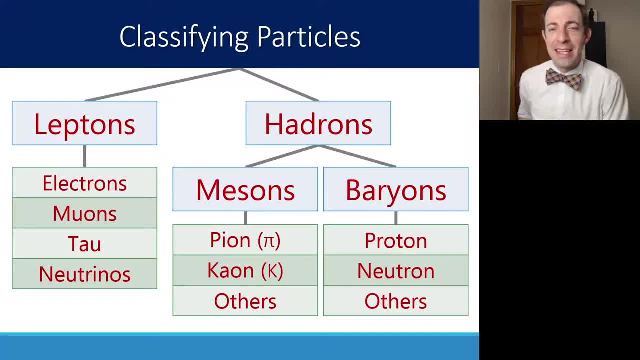 neutrons, as well as several others that are in that list. While mesons are made out of two quarks, baryons are made out of three quarks, But all of these are under the umbrella of hadrons, which are particles made out. 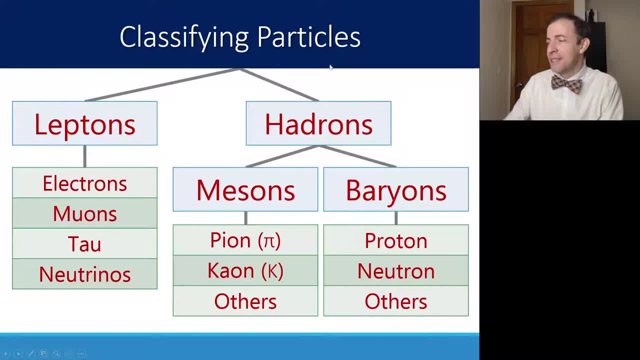 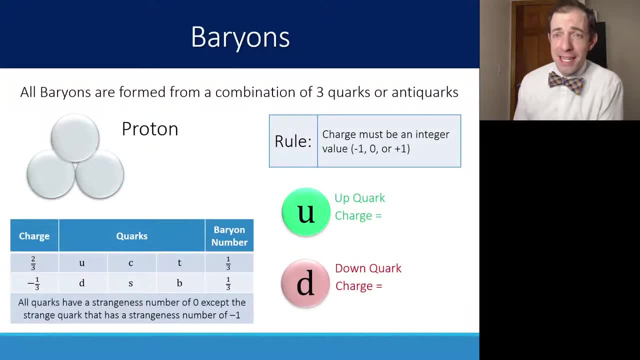 Of quarks, either two or three, So leptons or hadrons. hadrons can be mesons or baryons. Now let's look at baryons Specifically. let's focus on the proton and the neutron, because these are baryons that we use all the time. They are in every atom that we have, And it is important. 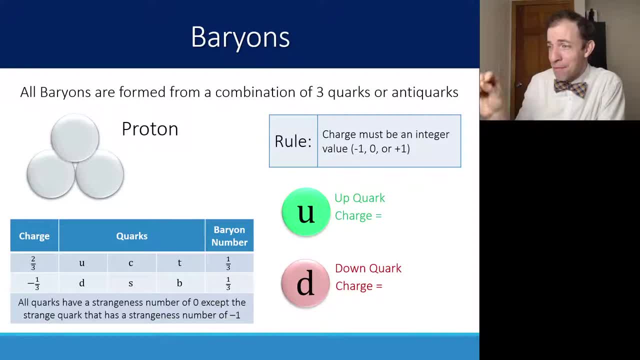 for us to know how these baryons of protons and neutrons are comprised in their quarks. Well, the most common quarks are up quarks And down quarks, And this is what protons and neutrons are made out of. Now, if you look at, 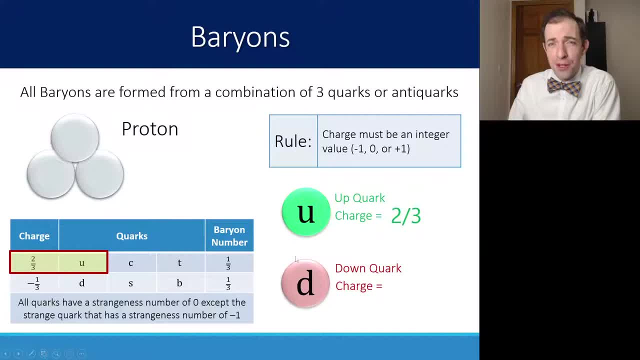 your table. here, you'll see that the up quark has a charge of two thirds and the down quark has a charge of minus one third. Now, with that as our possible combination, our rule is that the charge will always end up being an integer, That's negative one, zero or positive one. We 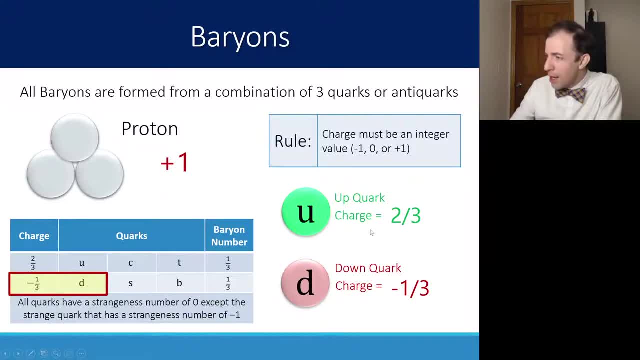 know that a proton has a positive one charge And if you look at up and down you can probably figure out if there are protons and neutrons that are made out of protons and neutrons. And if you are going to be three quarks total, how does it need to be situated so that the up quarks and the 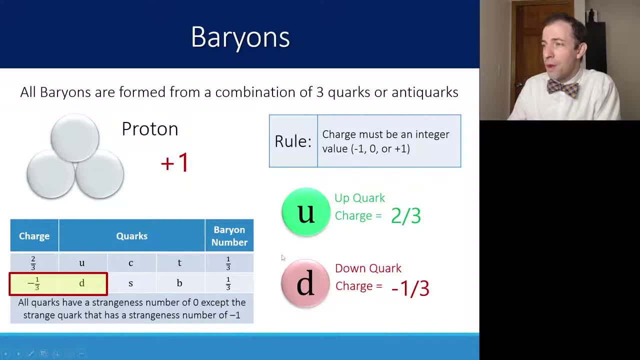 down quarks leave you with a positive one charge. Well, one of the quarks is an up quark That gives me two thirds. If I have another up quark that gives me four thirds. And then a down quark brings. 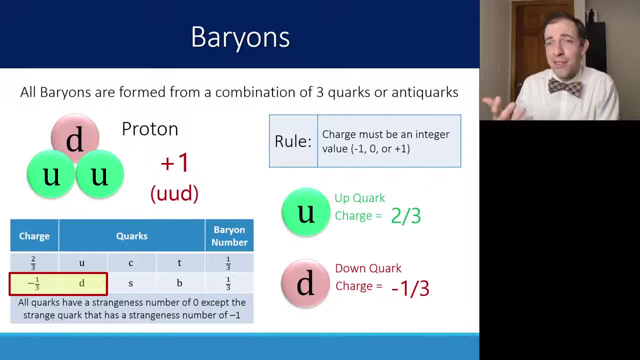 that down to three thirds, which is a plus one charge. So we have an up up down. Sometimes we can draw it like this as a group of three quarks, Or sometimes you might see it just represented in parentheses: UUD. up, up down is the quark combination for a proton, For a. 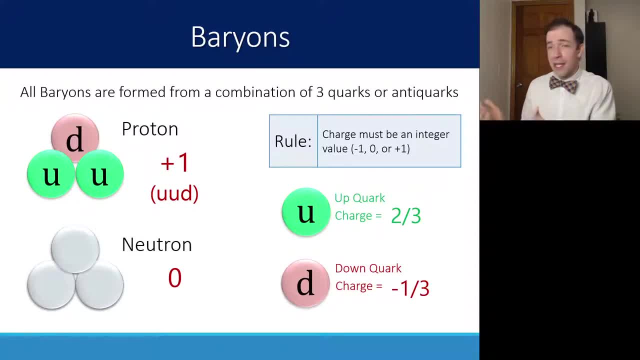 neutron. we know that that is a neutral charge. So likewise you can probably figure out the combination of up and down quarks to make that neutral happen. Well, here we have a down quark, a down quark and an up quark, So two thirds and then minus one third, minus one third. 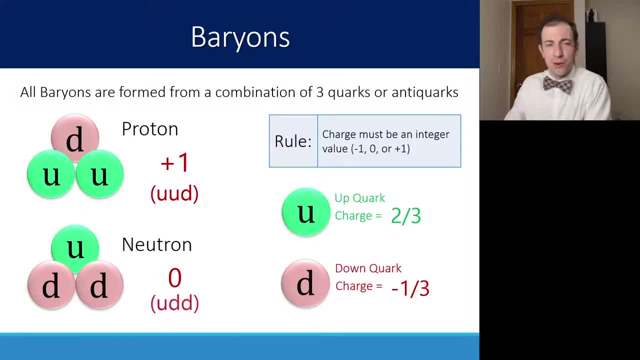 brings us down to zero for our neutral neutron. That is a UDD or up down down configuration. So again, these are both baryons because they're made out of three quarks. Let's look at some mesons. These mesons are always going to be formed with a combination of quark. 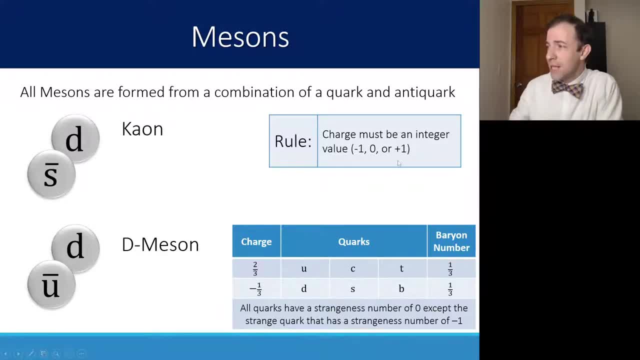 and an anti-quark, because the rule always stays the same here that you must have an integer value, negative one, zero or positive one. So if I look at this kaon, here I've got a down quark And again this bar on top means it's an anti-strange quark. Well, I find on my list down quark is a. 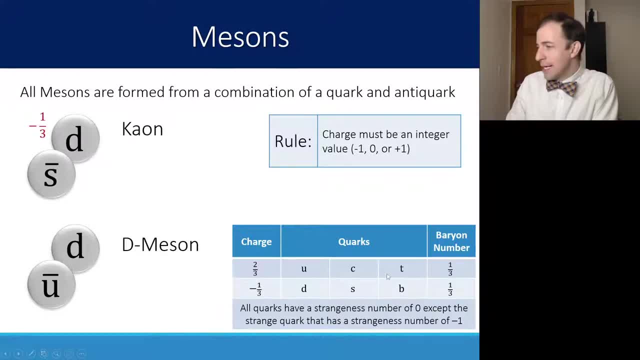 negative one third. So I'm going to look at this down quark and I'm going to look at this down quark And again, this down quark is a negative one third charge. Then I find strange is here. Well, strange says it's a negative one third, but since it's an anti-strange, that becomes a. 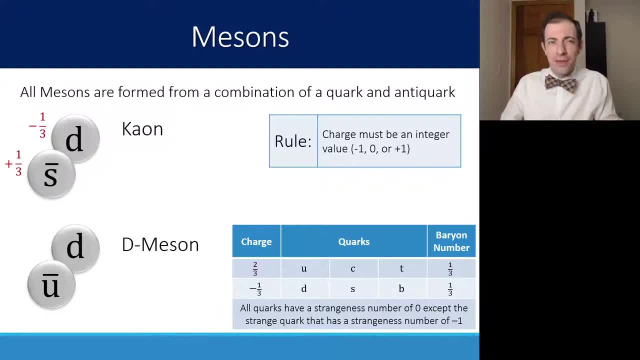 positive one third. So I have a negative one third, positive one third. they cancel each other out and we have a charge of zero. Now we can do the same thing for a D-mason. A D-mason is a down quark and an anti-up quark, So we can figure out what that charge needs to be The down quark. 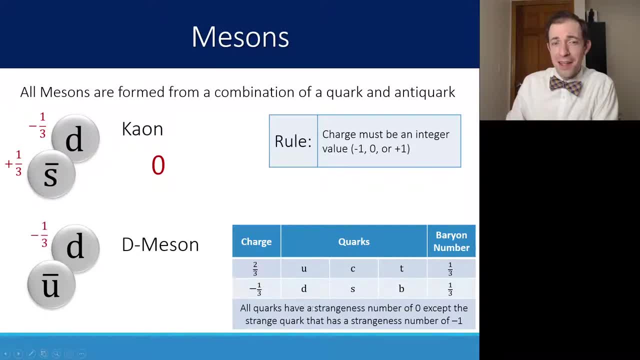 again, here is a negative one third. An up quark is a two thirds, but it's an anti-up quark which makes it a negative two thirds. So my D-mason, I can predict, will have a charge of minus one, And we can do this with any. 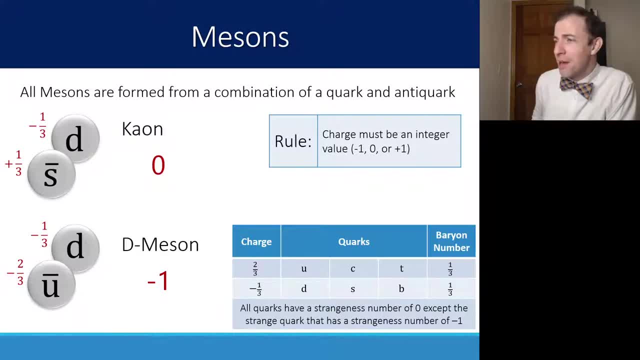 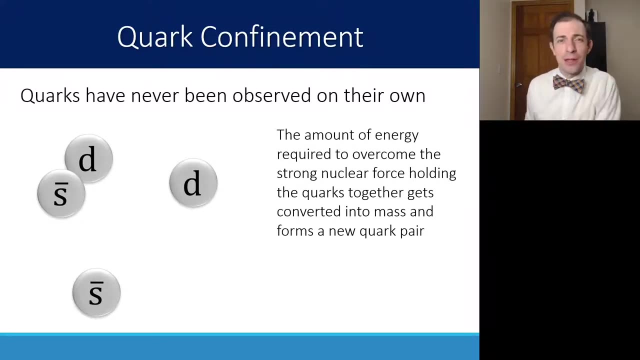 mason or baryon that's given to us, because we can use this table to help us identify what the charge of the individual parts are going to be, which can help us figure out the charge of the whole. All right, so we've seen these two quark combos, or these three quark combinations. 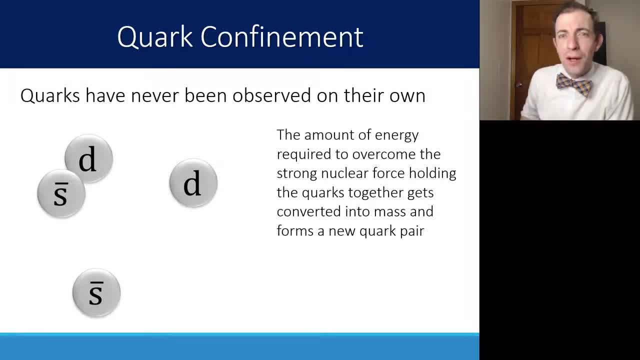 well, what about one quark combinations? Well, it turns out that quarks have never been observed on their own. This is a phenomenon known as quark confinement. And you might think, okay, well, let's take a mason which only has two and let's rip those quarks apart. Let's add energy so that. 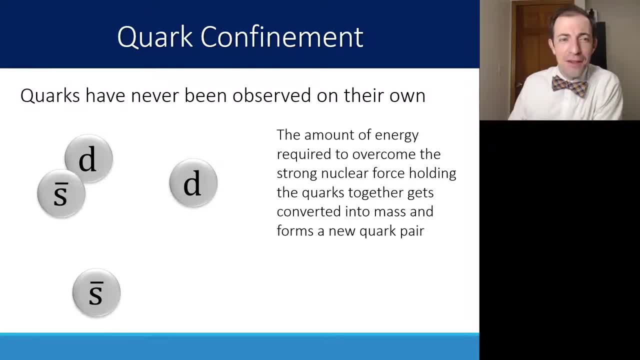 the quarks are no longer together. Well, it turns out that the amount of energy required to overcome that strong nuclear force that's holding those together is actually enough energy to be converted into mass. So if you were to add enough energy to separate the quarks, well too bad, because that energy was 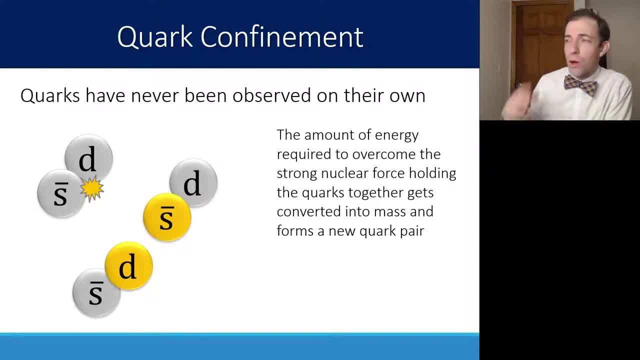 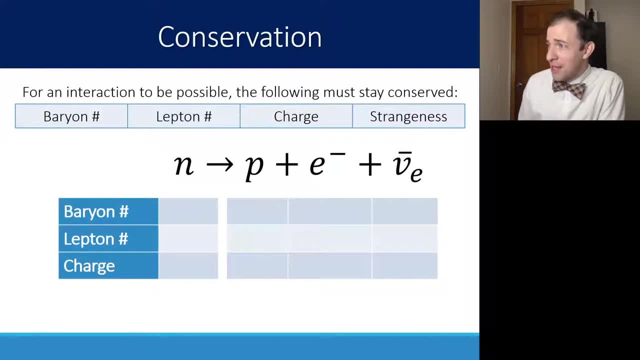 converted into mass and you have two masons now instead of one. So quark confinement means that quarks will never be found or observed on their own. And then another thing that we'll need to be able to talk about in these particle interactions will be conservation We're familiar with. 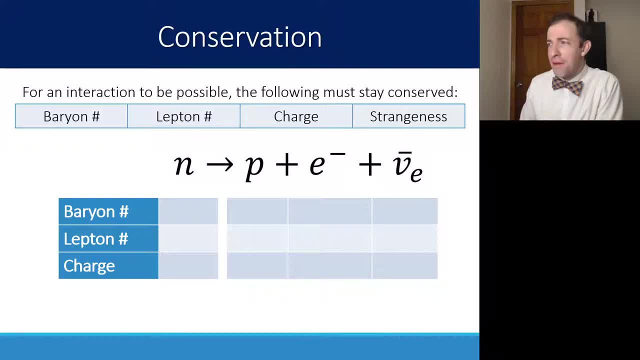 conservation in chemistry, conservation of mass, You might be familiar with. our conservation is conservation of momentum or conservation of energy. We've talked about that in physics as well. But here there are some different properties that are always conserved in the world of particle. 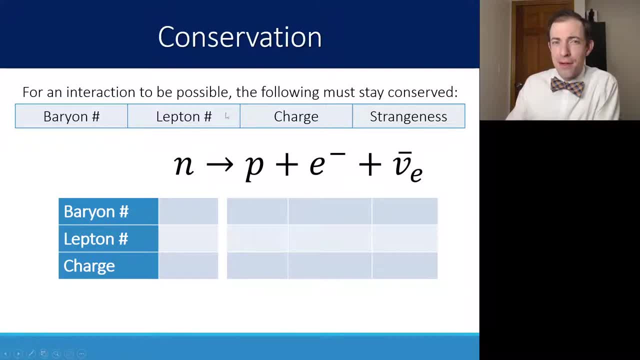 physics, And the properties are baryon number, lepton number, charge and strangeness. Strangeness will really only ever apply if there are strange quarks in here. So we're not going to see strangeness here in these slides, but you might encounter them later on. Let's focus primarily. 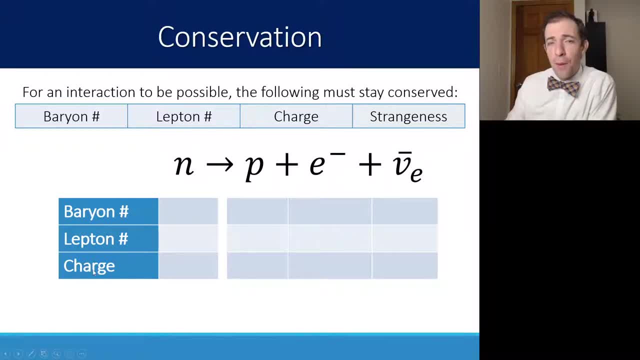 here on baryon number, lepton number and charge. So we're not going to see strangeness here in this slide. Let's focus primarily here on baryon number, lepton number and charge. Well, if I see my 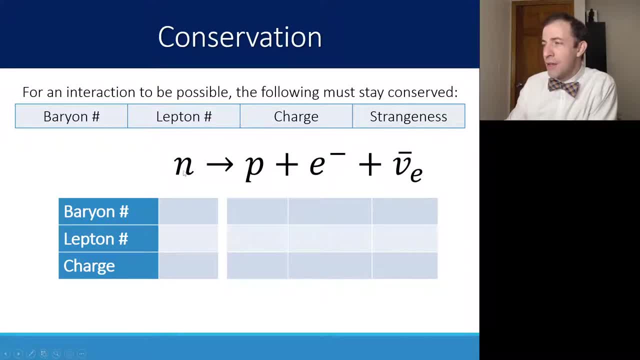 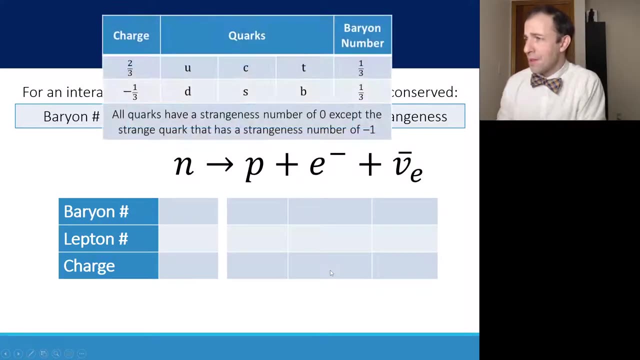 particle interaction presented as is here. I have a neutron which turns into a proton, an electron and an antineutrino. That might feel familiar. That is the process that kind of underlies the beta negative decay that we talked about earlier on in the unit. Well, if I look at my list of quarks, 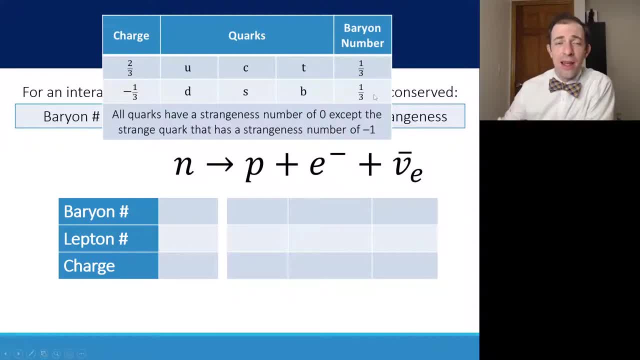 I see that baryon number shows up in that list And every quark has a baryon number of one-third And an antiquark would just have a negative one-third baryon number. Well, here I know that a neutron is made out of three quarks, So three times one-third will give me a baryon number of. 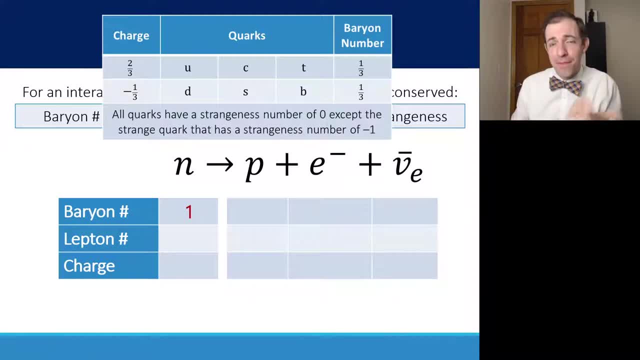 one. Any baryon number will have a baryon number. or any baryon has a baryon number of one. A neutron is A proton. here same thing. three quarks gives me a baryon number of one: An electron and an. 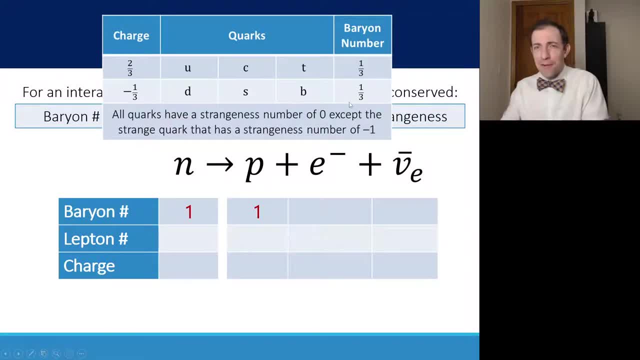 antineutrino are not quarks. They're not made out of quarks. They do not have a baryon number of one. They do not have a baryon number at all. So they are both zero for their baryon number. 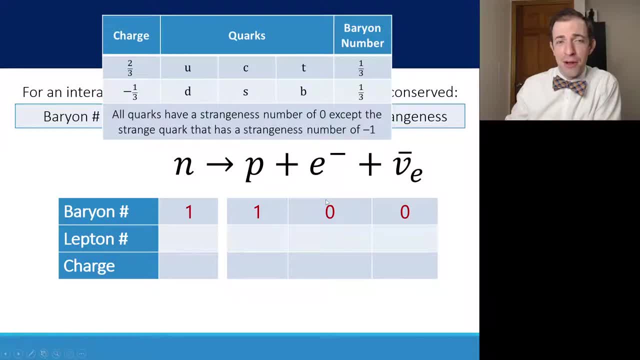 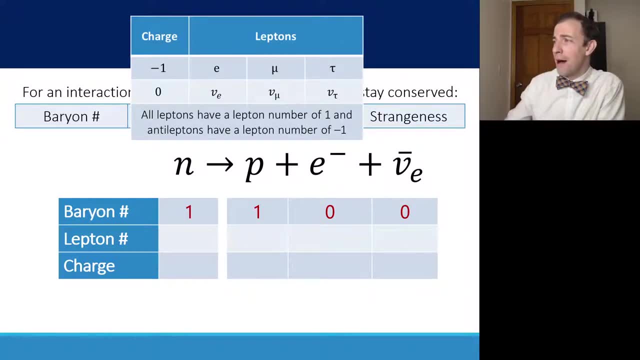 Baryon number is conserved. I have one on both sides of that particle interaction. Next, let's look at a lepton number To find that. I need to look at the lepton table on my data booklet. Here all leptons have a lepton number of one and anti-leptons have a lepton. 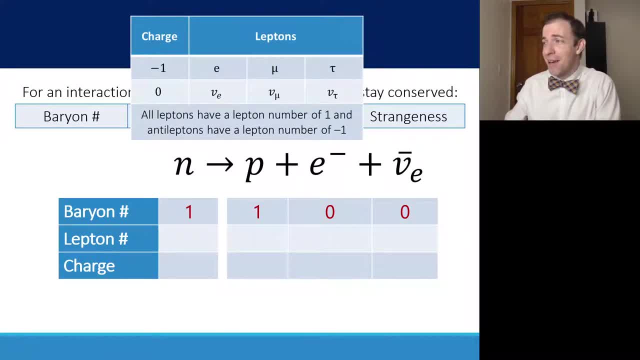 number of negative one. Nothing said there about anything made out of quarks. Neutrons and protons have no leptons associated, So an electron here is a lepton that has a lepton number of one, and this antineutrino is an anti-lepton, which means it has a lepton number of negative one. 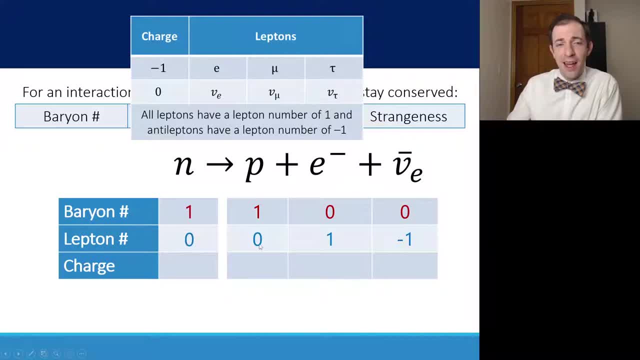 Lepton number is conserved, I have zero on the left-hand side, and then zero plus one minus one, which gives me zero as well. All right, my last piece here is the charge Charge. we know for neutron is neutral, That's zero. For a proton, we know that's positive one. 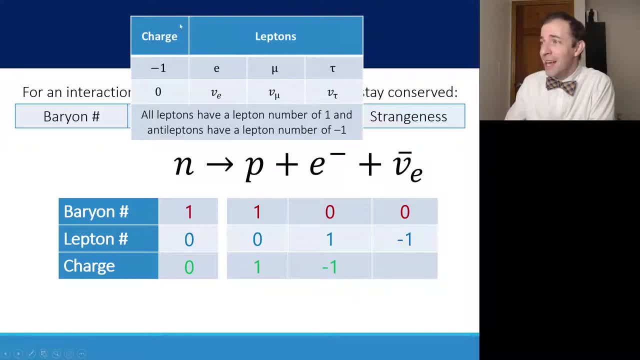 For an electron, we know that's a negative one. And then here you can look at these other leptons, this antineutrino. It doesn't matter if it's a neutrino or antineutrino, It will have a charge. 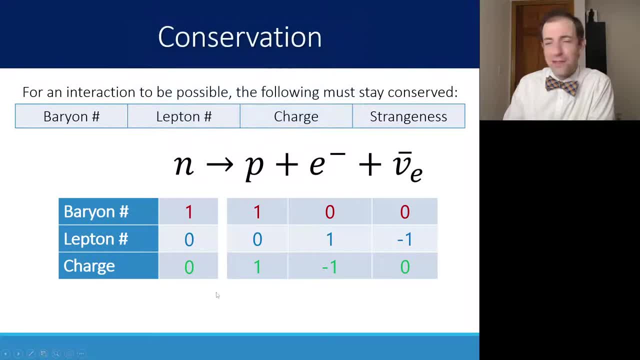 of zero. Again, charge is conserved, just like these other numbers were. Zero turns into one minus one plus zero. So this interaction is valid because all of these properties are conserved. Now let's look at a couple more examples. 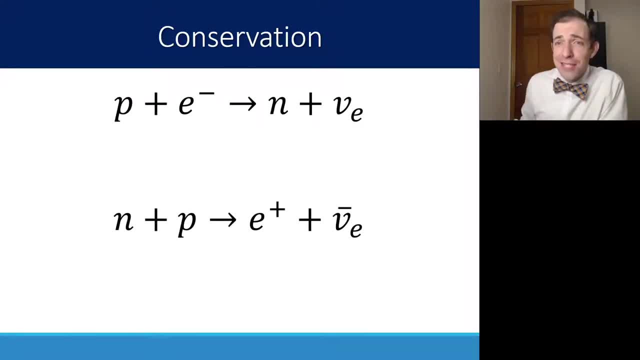 If I give you two more situations here, you can look at each of these numbers and see if these numbers are conserved. You may not recognize the configuration of the things that are shown, but looking at conservation, even if you're not familiar with it, you can determine. 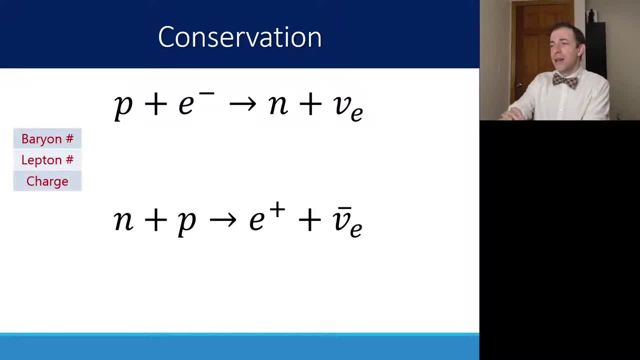 is this valid or is this not valid? Is this something that could happen or not? So again, here are the three different properties, ignoring strangeness number for now, that we're going to keep trying to conserve. So if we look at the left side, 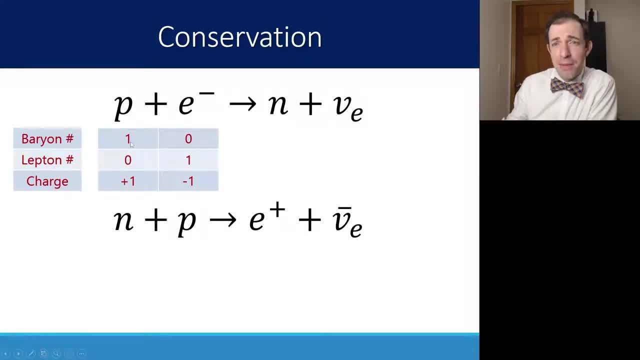 of this interaction. proton has a baryon number of one, a lepton number of zero and a charge of plus one. This electron has a baryon number of zero, a lepton number of one and a charge of minus one. All right, Now the right-hand side, my neutron. 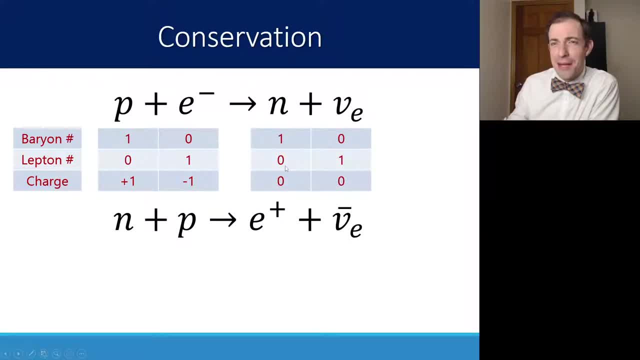 is a baryon number of one lepton number of zero because it is not a lepton and a charge of zero because it is neutral. And then my neutrino is a baryon number of zero because there are no quarks. 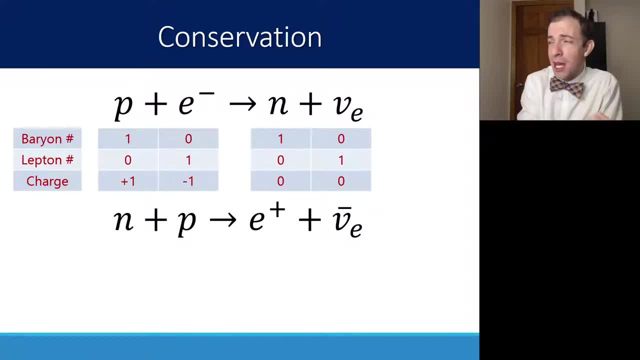 A lepton number of one, because it's not an anti-neutrino like we saw before, and then a charge of zero. Everything seems to be conserved. Baryon number is one on both sides, Lepton number is one on both sides and the charge neutralizes to zero on both sides. So yes, 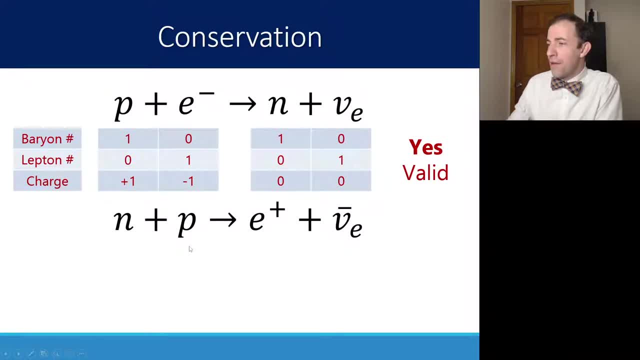 that is a valid particle interaction. Now, if I look at this one down below, I've got a neutron and proton. Those are both baryons and not leptons. So baryon number one and one Lepton number is zero and zero, And then the charge is neutral for the neutron. 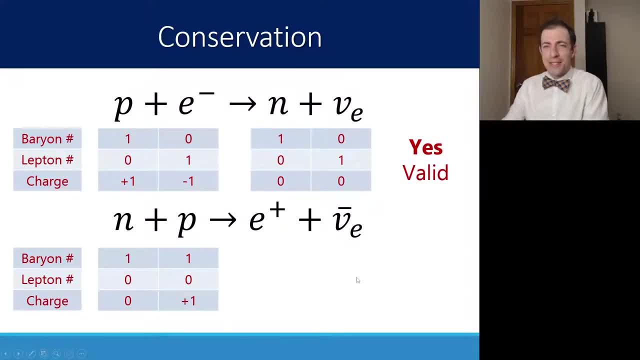 and positive one for the proton. All right, I'm going to look over. on the right-hand side, I've got a positron which is an anti-electron and an anti-neutrino. That means that their baryon number is zero for both of them. There's no quarks. 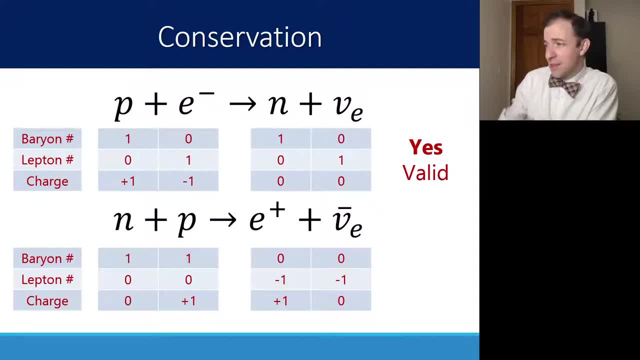 Their lepton number is negative one because they are both anti-leptons, Even though we don't see the bar over the top of this positron. it is an anti-electron, which is another way of writing that, And that means we have a charge of plus one and a charge of zero. It looks like charge is. 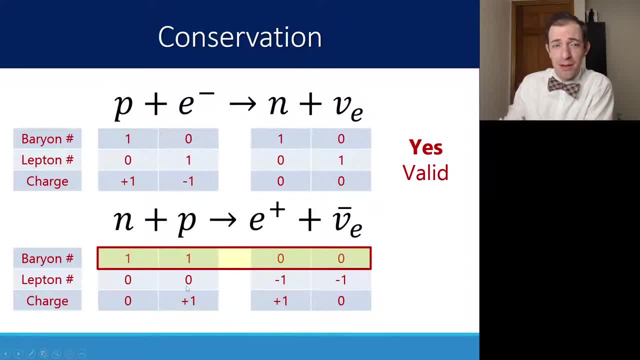 conserved, but baryon number is not. We have two and zero, and lepton number is not zero and negative two, So this is invalid. These particles cannot interact in this way because these properties are not being conserved. All right, The final type of particle that shows up in our 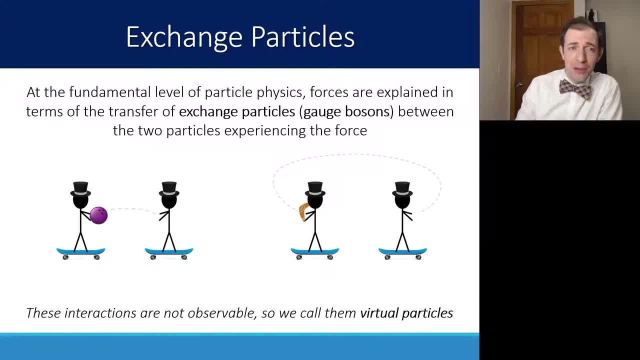 model is something called an exchange, particle Exchange. particles are ways that we can explain force in terms of particles. So the particle model, the standard model, means that everything is made out of particles or can be explained in the form of particles. Well, force is one of those. 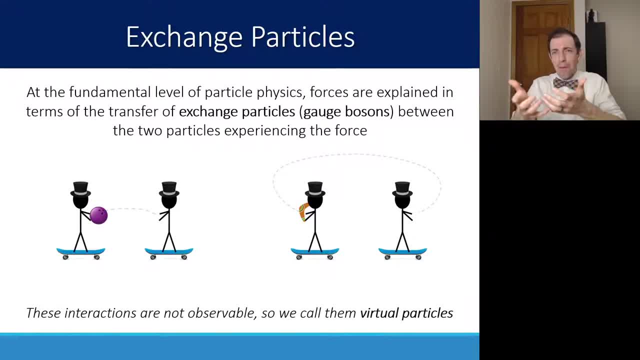 weird things to try to explain as a particle. If two things are being repelled, how is a particle doing that? Well, there are a couple of different conceptual models that can help us understand that. Imagine that we have this particle, this bowling ball, giving us this force of repulsion And 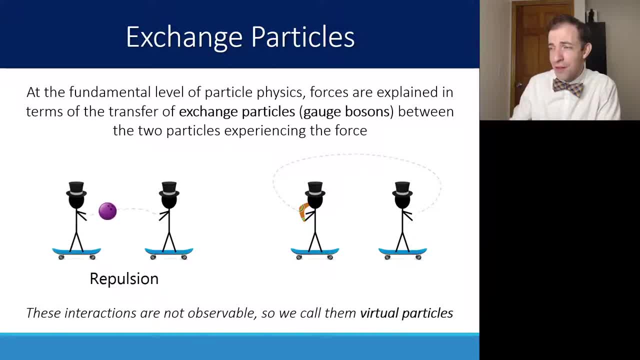 imagine that that bowling ball is just making the rounds going back and forth. When it leaves one particle, it kind of sends it out, When it's caught by another particle it sends it backward. And if that bowling ball keeps going back and forth, you can imagine these two skateboarders. 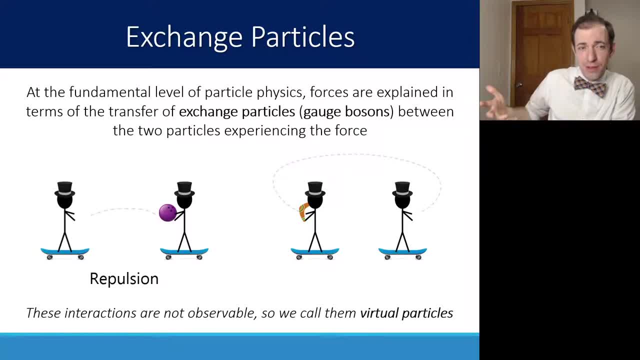 drifting apart farther and farther. that force of repulsion. Now here to get a force of attraction is a little bit harder. It's kind of a stretch. But imagine, instead of a bowling ball we have a boomerang, So it's being thrown opposite. 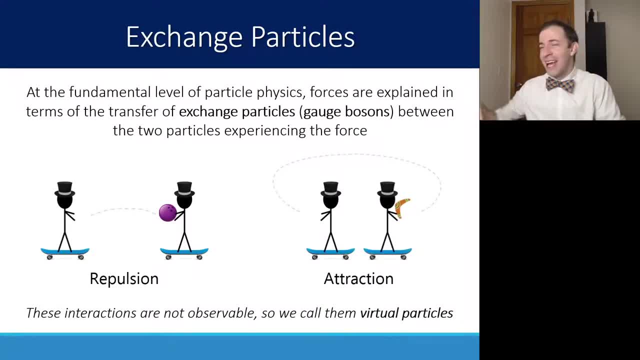 kind of going back and around and being caught opposite. And each time it's thrown and caught, those skateboarders get a little bit closer together in this form of attraction. Well, these interactions, they're not observable. We don't see these particles going back and forth. 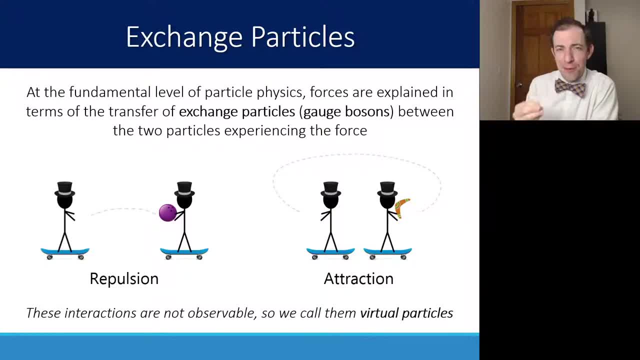 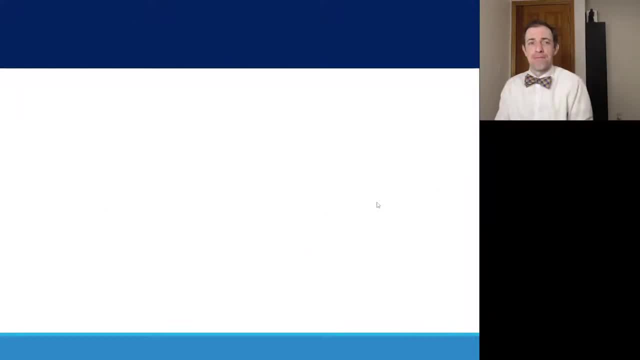 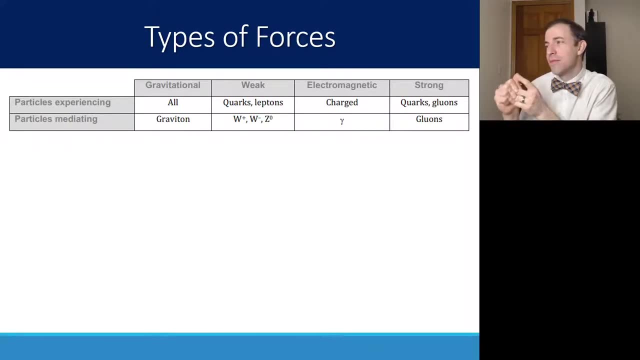 We call these virtual particles. It's a way of describing forces. Everything can be described in this form. It's a form of particle nature. All right, These four forces that we've seen before- gravitational, weak, electromagnet and strong force- are the four fundamental forces. You'll see that each of these 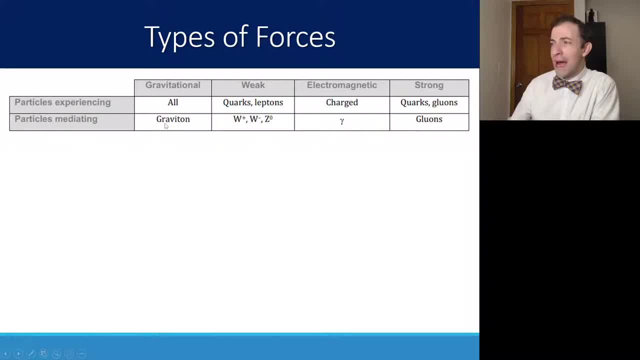 have mediating particles. The gravitational force, we call the mediating particle a graviton. The weak force has a few different particles that we'll see in the next lesson: The W plus, W minus and the W minus. So we'll see that in the next lesson. So we'll see that in the next lesson. So 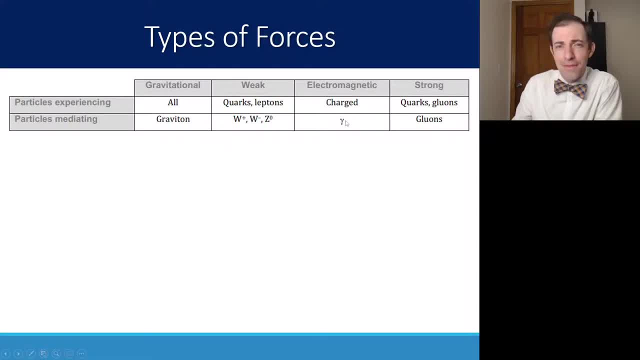 Z naught Electromagnetic has this gamma, that is our symbol for a photon. And then strong nuclear force is gluon, sticking the protons and neutrons and any baryon or hadron together. Now these are arranged in the data booklet in order of weakest to strongest. Strong is our. 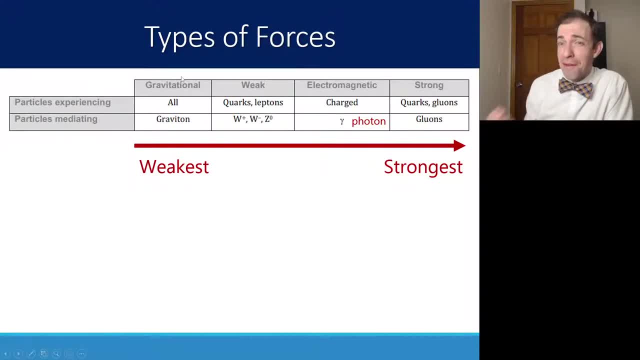 strongest, go figure, And gravitational is actually by far the weakest force, which is weird because that's the force that we seem to experience in our own lives the most, but it is by far the weakest. It's weak enough that you can actually overcome it by simply jumping. You are 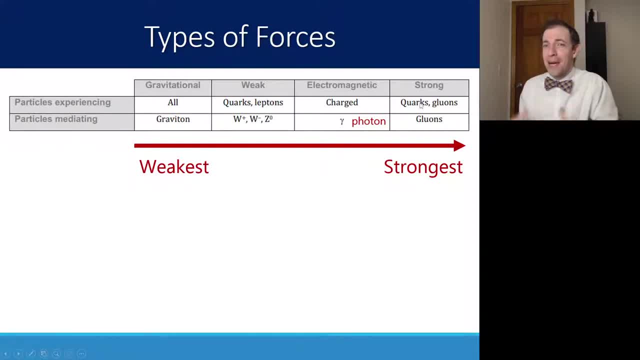 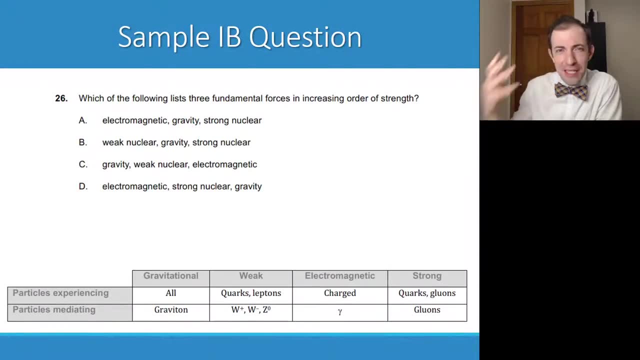 not going to be able to overcome something like this strong nuclear force by any force that you are able to impart. And every once in a while Ivy will ask a question kind of surrounding these ideas. which of the following lists three fundamental forces, in increasing order of: 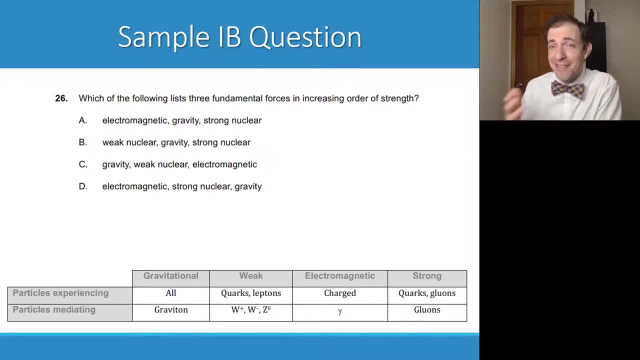 strength. Well, if you know that the data booklet gives it to you in this increasing order, you can pretty clearly find the answer. In this case there's only three different examples that are shown, but gravity, weak, nuclear and electromagnetic are in the correct order left to. 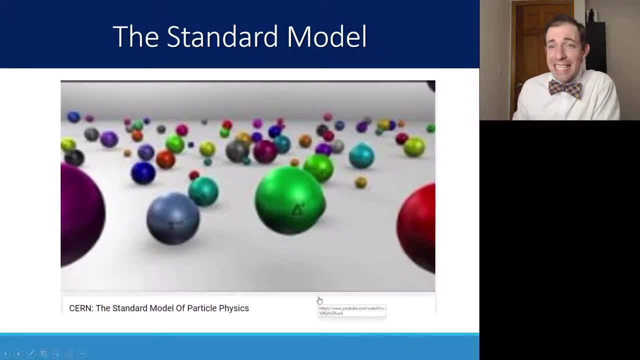 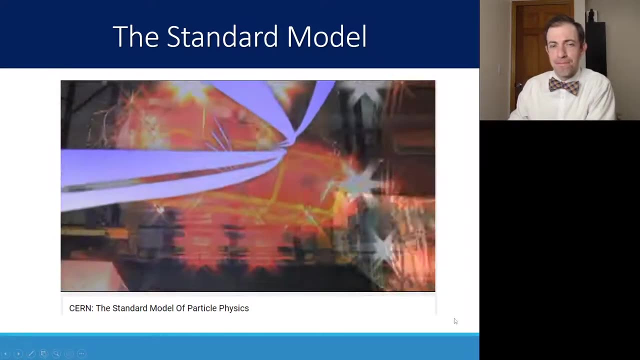 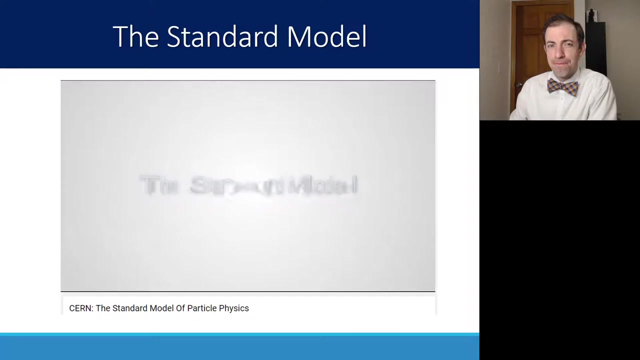 right, All right. that leads us to trying to summarize and understand all of these things together, And we do so in something called the standard model. The objective of particle physics is to understand the basic structure and laws in nature all the way from the largest dimension in the universe- formation of galaxies and stars. 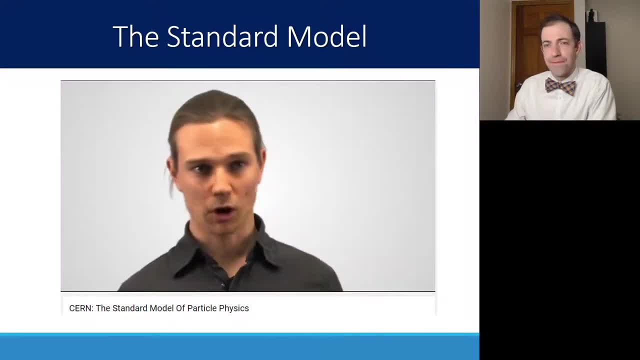 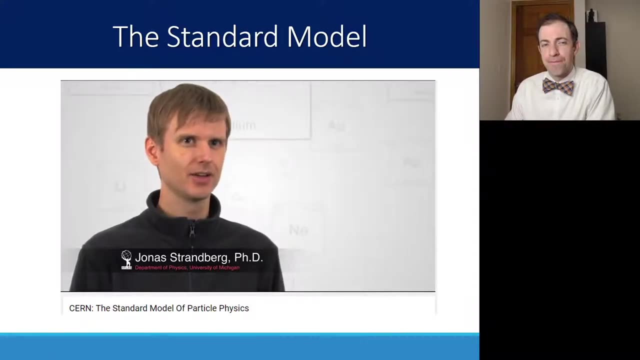 all the way down to the smallest dimension in the microcosm. So historically, we knew about all of the different elements in nature. We knew about helium, hydrogen, oxygen, gold, lead and so on, which are all made of different atoms. 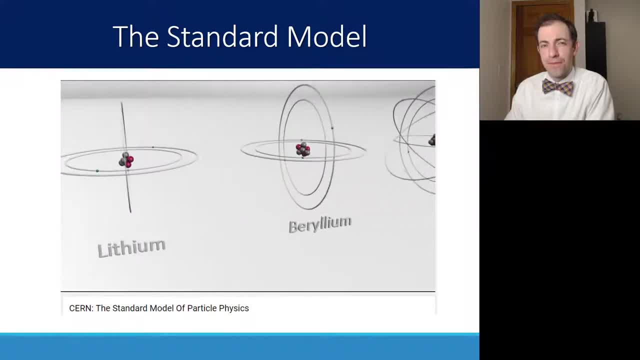 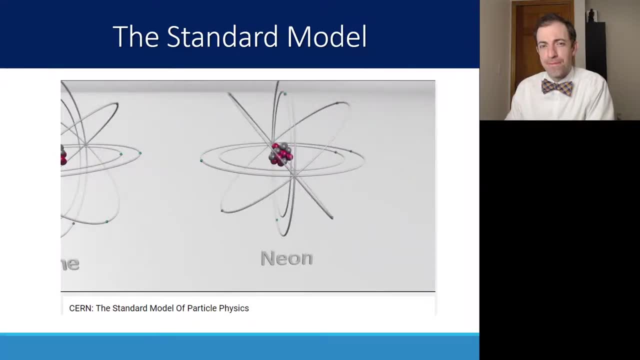 But a great simplification was made when we realized that all the atoms are just made out of three particles: the protons, the neutrons and the electrons. And just by adding more protons, more electrons, we get a different element, a different type of atom. 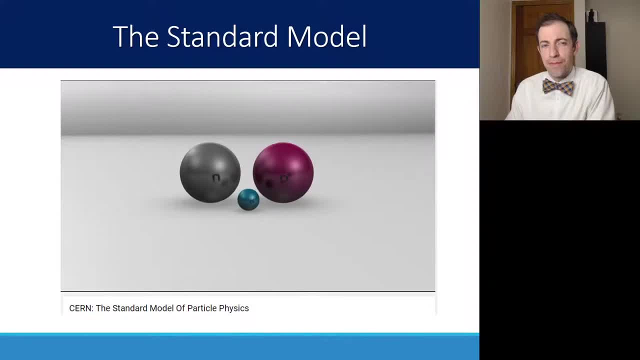 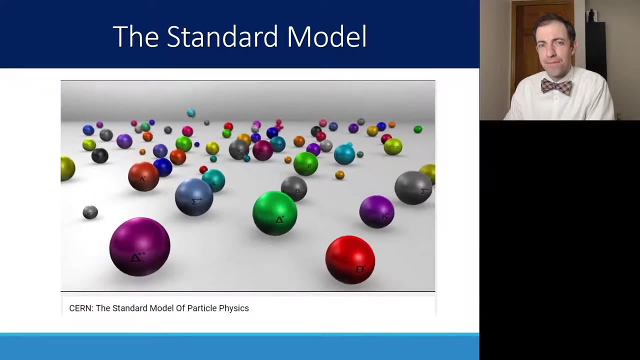 In principle we can build a very simple universe with just protons, neutrons and electrons. But it became much more complicated in the beginning of the 20th century when we found many, many new particles from cosmic rays. There wasn't really a system established to organize this zoo of particles. 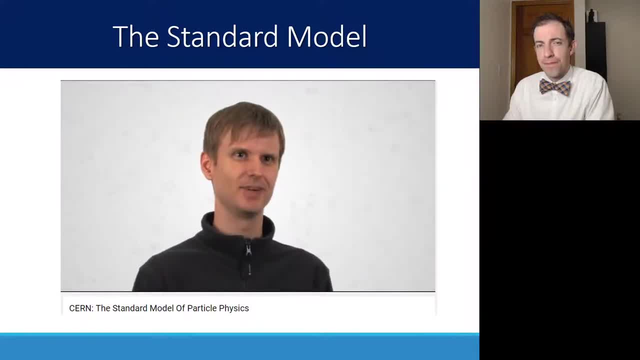 So we were calling these new particles things like pi, sigma, delta and so on. And things got so bad we were running out of symbols to name these particles. So we started organizing these particles according to the properties they have, And the properties are things like spin, electrical charge. so if they're positively charged, 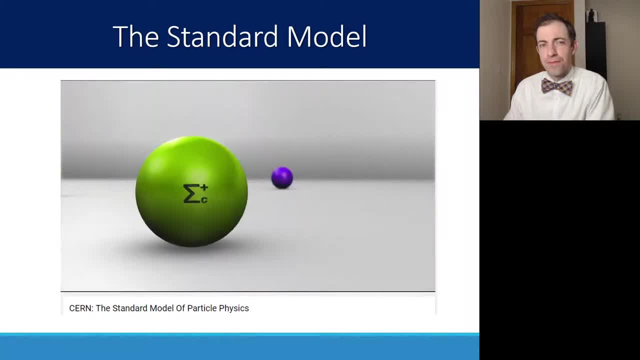 negatively charged or neutral mass of the particles and the lifetime of the particles, which is how long it takes before they decay into lighter particles. To simplify the picture, new fundamental particles called quarks were predicted, And the whole zoo of particles could be described by combinations of these quarks. 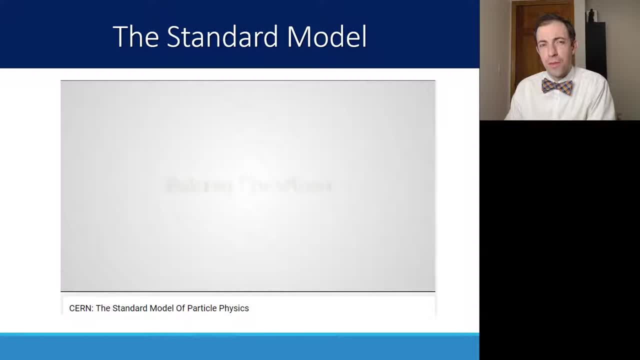 And this was the birth of the Standard Model. At the beginning, there were only three quarks. Then a fourth, fifth and sixth quark was predicted and then discovered, and this gave us great confidence in the model. In addition to these quarks, there's another set of fundamental building blocks of matter. 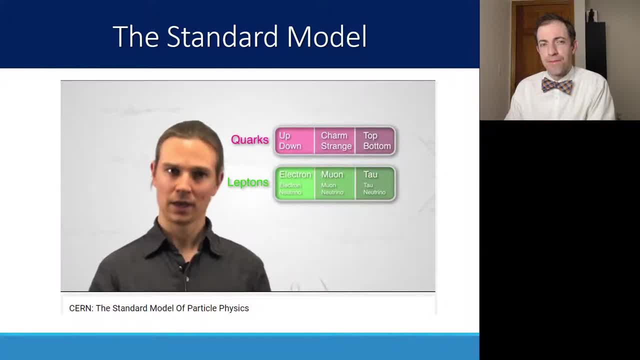 the so-called leptons. They are composed of an electron, their heavier cousins, the muon and the tau- and this is a physical particle- and their neutrino partners. In addition to the fundamental building blocks of matter, the standard model also incorporates: 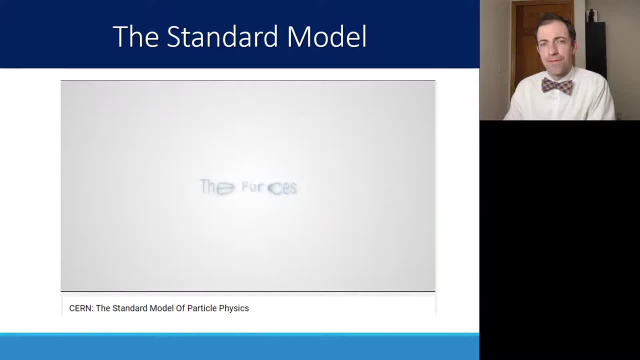 the fundamental forces. The exchange particles of the weak force are the W and the Z bosons. The weak force explains the energy production in the sun and is responsible for the radioactive beta decay. The electromagnetic force acts on charged particles. The corresponding force carrier is the photon. 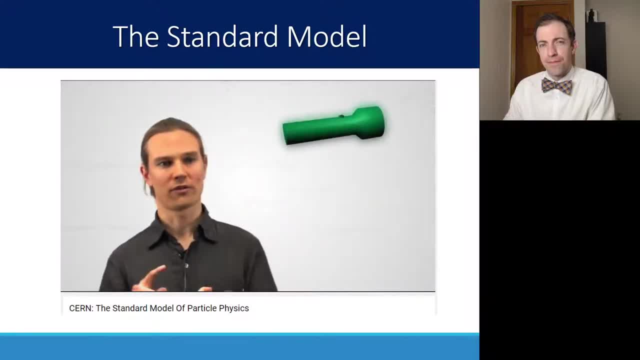 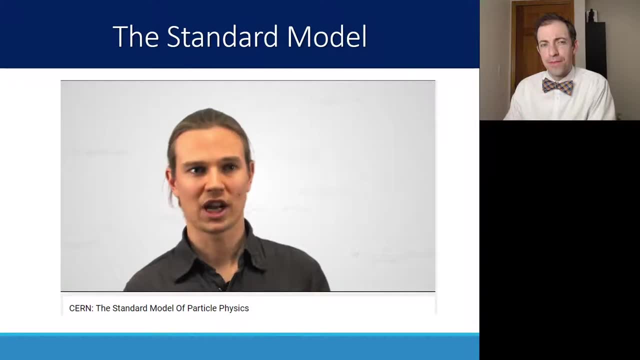 The electromagnetic force is responsible for propagation of light or for the fact that a magnet can pick up a paper clip. The strong interaction acts on the quarks. The corresponding force carrier is the gluon. The gluon literally glues together the quarks in the neutrons and the protons and it holds. 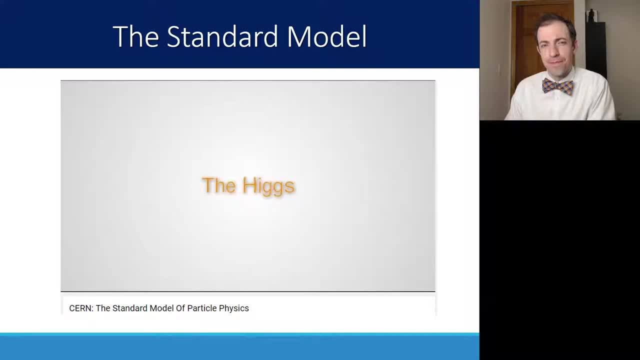 the nucleus together. Understand? Yeah, The standard model is extremely successful and it has predicted all the phenomena we have seen so far at the microscopic level. This is a beautiful theory. It is self-consistent, It's predictive, But it's incomplete. 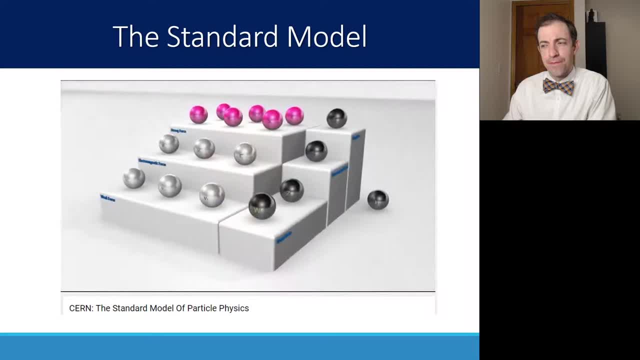 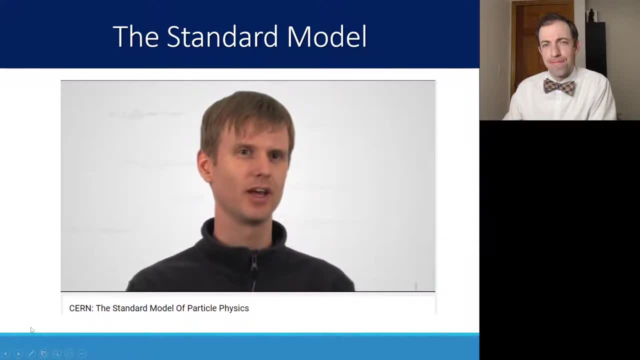 There's one last missing piece of this puzzle, and that's the Higgs program. It's the holy grail of particle physics. We know exactly what it should look like and we have predicted this particle since over 40 years and we use it in all our calculations and so on. 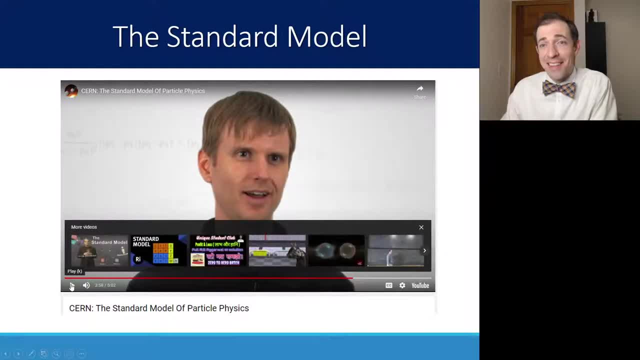 We're pretty sure it's there, But we haven't figured it out. We haven't found it so far. All right, That's where we'll stop that video, because in the next lesson we will talk about the Higgs boson, because since the creation of this YouTube video it has been discovered. 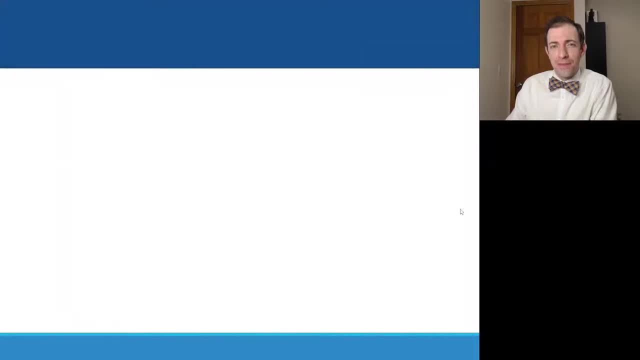 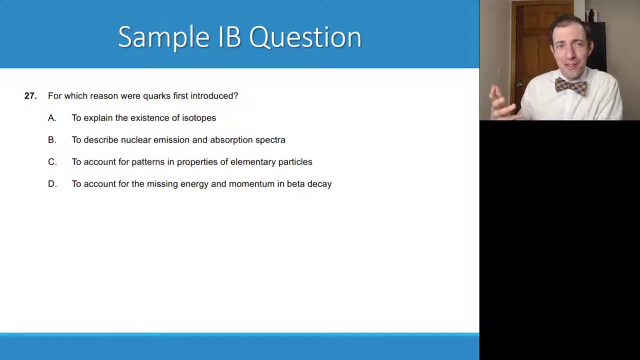 and measured in the Large Hadron Collider. So a sample IB question just to understand, kind of, the creation of this standard model. For what reason were quarks first introduced? Well, one of the things that they described very well in that video was basically the. 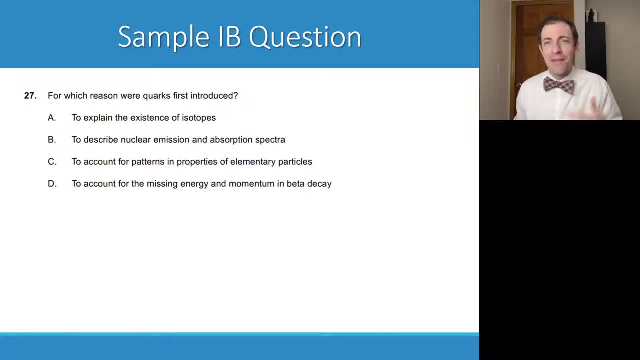 quarks. They were the only kinds of quarks that were possible in the world. So they were the only kinds of quarks that were possible in the world. So the theory of quarks is that quarks are just different from quarks. 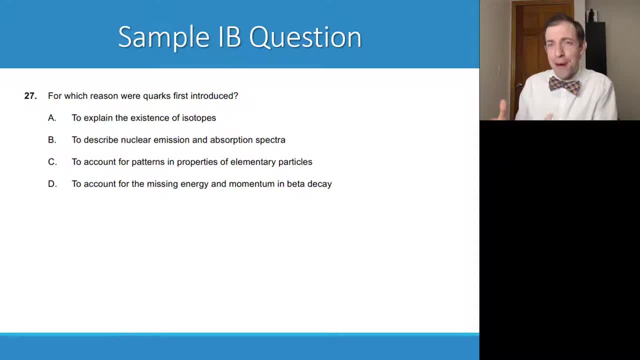 They're not exactly the same as they are. They're just different in nature And they're also different from other things. So what we're trying to do is try to find patterns, just like Mendeleev and other scientists around the time of the periodic table used that to better understand these other patterns.